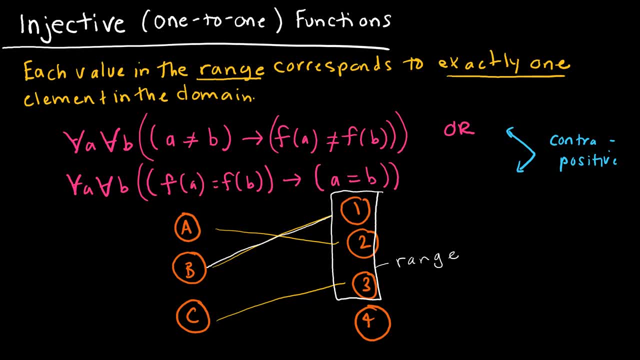 1 corresponds to only B, 2 corresponds to only A, 3 corresponds to only C. If, however, I were to add an element D in my domain- remember, this side is the domain- if I were to now add an extra element D and that element mapped to 3, this is no longer a one-to-one function. 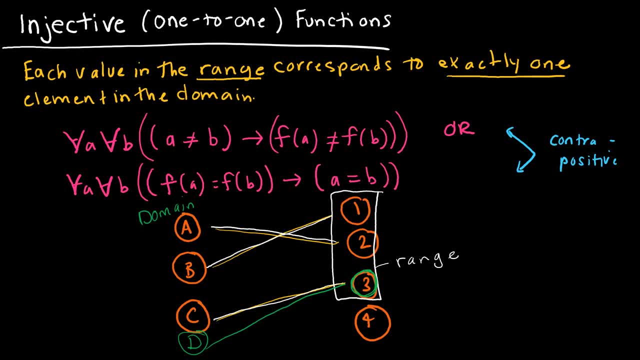 because this value in the range, this value in the range, maps to 2 elements in the domain and therefore it would not be one-to-one. So let's take a look now at what these two statements say. These two statements are saying: 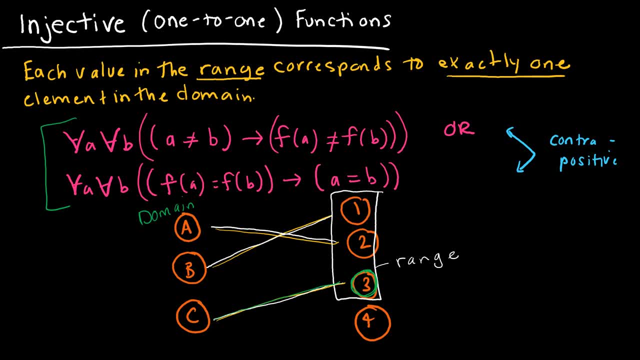 the exact same thing. they're just contrapositives of one another. The first says: for all A and for all B if A does not equal B. so let's just use A and B here if A does not equal B. 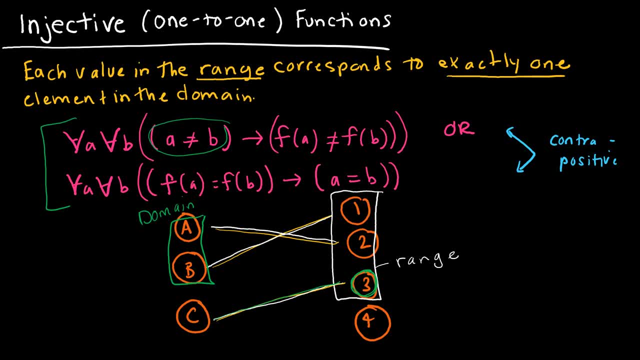 which they are not the same element. that implies that that element is a one-to-one function. If they were an equal element, there would be no difference between a and b. Therefore implies that f of a, in this case two, does not equal f of b, in this case one. That's exactly. 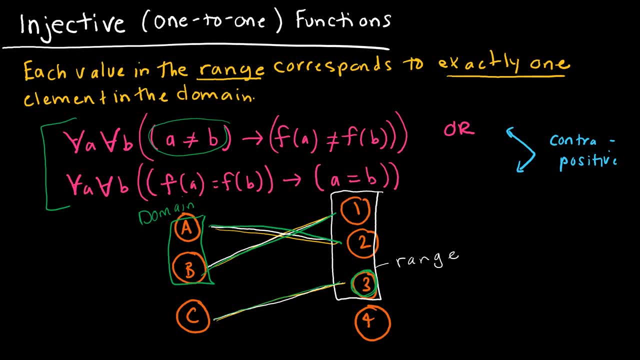 what it means to be a one-to-one function. A does not equal to b, and therefore their outputs are not equal as well. Or if you have f of a equal to f of b, so if we have some value in the range that's equal to itself, essentially, then the values that map to it must be the same. 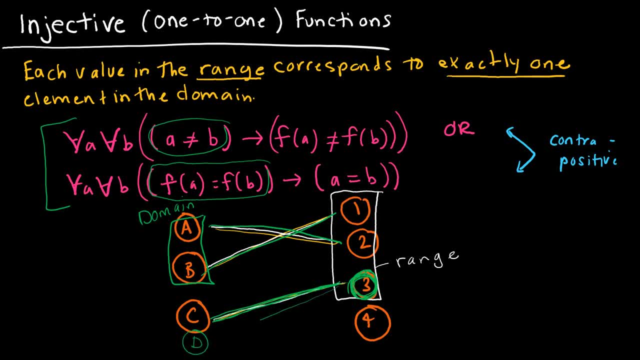 So that's why it didn't work when I had this d here, because if three is equal to three, but f of c equals three and f of d equals three, that violates this guy right here. So that is a one-to-one function. Let's take a look now at a surjective or onto function. 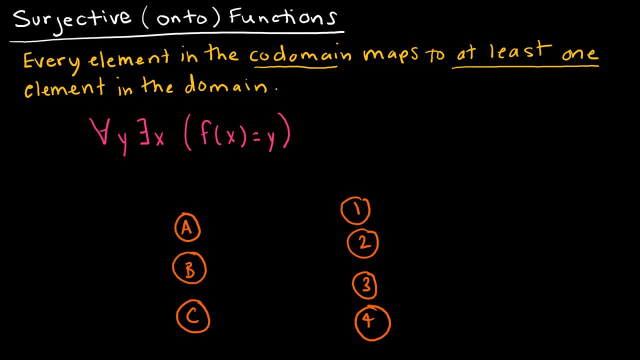 In a onto function, every element in the codomain maps to at least one element in the domain. So let's remember: this is domain and this is codomain. And let's say a maps to one and b maps to two and c maps to four. Now we just talked about one-to-one functions. 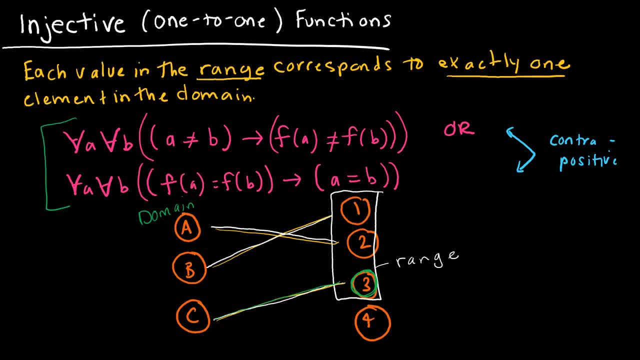 A is not the same element that B is using. The first element to be used is: let's compare the same thing for all A and for all B. So let's take a look at what these two statements say. These two statements are saying the exact same thing. they're just contrapositives of. 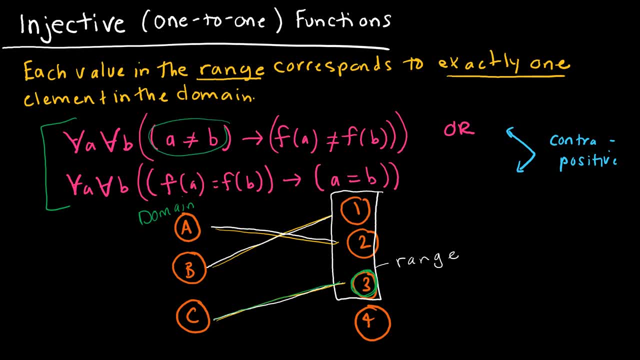 one another. The first says: for all A and for all B if A does not equal B, so let's just use A and B here. If A does not equal B, which they are not the same element, that implies that A is not equal B. 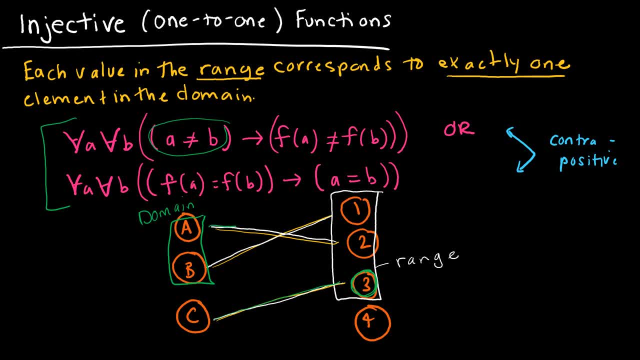 I'm going to give you a step back and see if that makes sense or not. that implies that f of a- in this case two- does not equal f of b, in this case one. That's exactly what it means to be a one-to-one function. 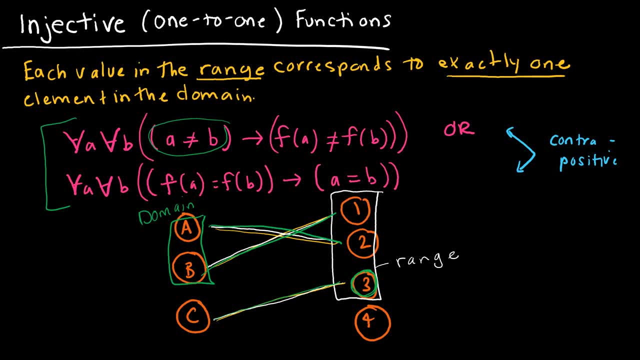 A does not equal to b and therefore their outputs are not equal as well. Or if you have f of a equal to f of b. so if we have some value in the range that's equal to itself, essentially, then the values that map to it must be the same. 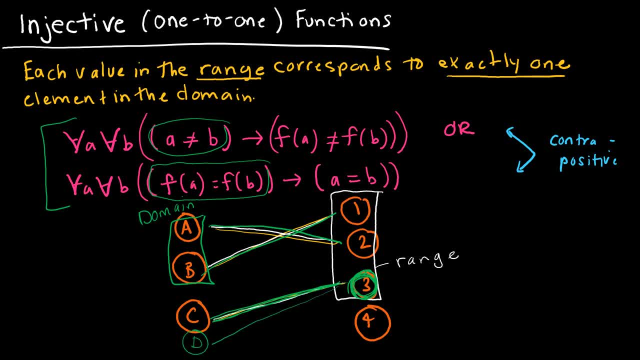 So that's why it didn't work when I had this d here, because if three is equal to three, but f of c equals three and f of d equals three, that violates this guy right here. So that is a one-to-one function. 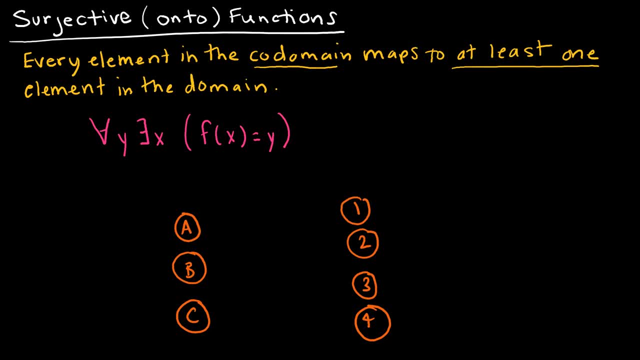 Let's take a look now at a surjective or onto function. In an onto function, every element in the context co-domain maps to at least one element in the domain. So let's remember, this is domain and this is co-domain. 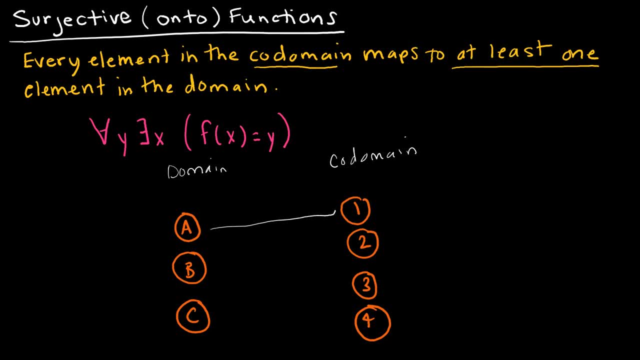 And let's say a maps to one and b maps to two and c maps to four. Now we just talked about one-to-one functions. This would be considered a one-to-one function the way I've drawn it now, because each element in my range and my range 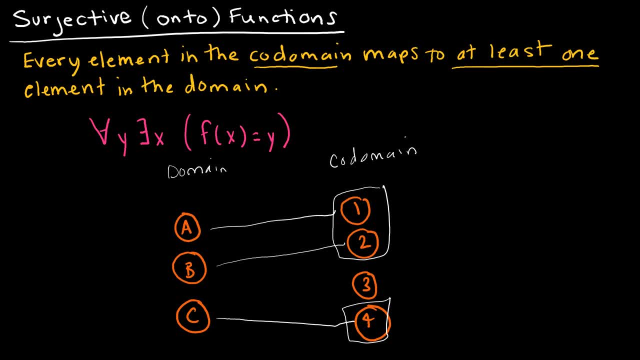 would be just the elements that are mapped to, has just one element mapped to from the domain. But that's not what we're asking. We're asking for a surjective or onto function. The onto function uses all values in the co-domain. 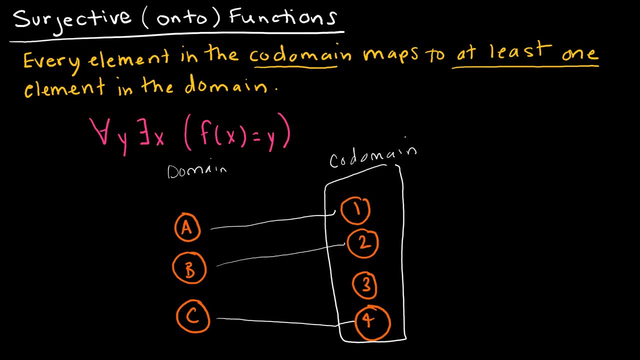 So the way I have it drawn right now, this is not onto, because three poor three is lonely and not mapped to by anything. So let's say I had some element d that maps to three. Well, now this is both one-to-one and onto. 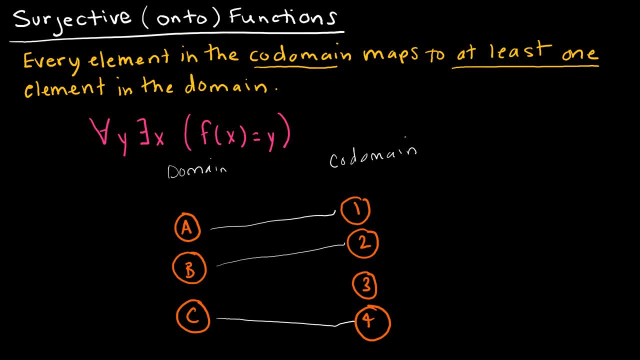 This would be considered a one-to-one function the way I've drawn it now, because it's a one-to-one function. So let's say a maps to one and b maps to two and c maps to four, Because each element in my range- and my range would be just the elements that are mapped to. 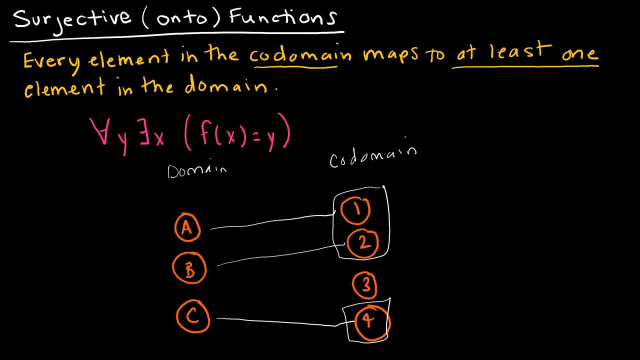 has just one element mapped to from the domain. But that's not what we're asking. We're asking for a surjective or onto function. The onto function uses all values in the codomain. So the way I have it drawn right now, this is not onto, because three poor three is lonely and 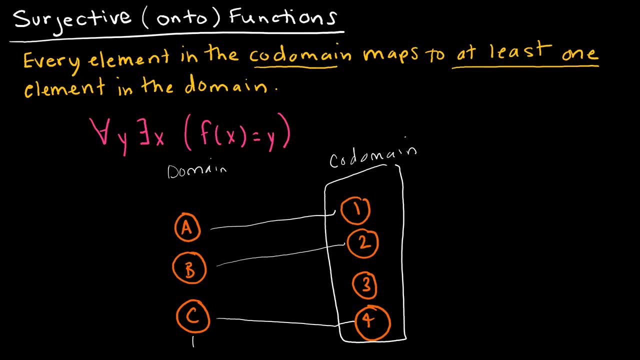 not mapped to by anything. So let's say I have a surjective or onto function and b maps to four. Let's say I had some element d that maps to three. Well, now this is both one-to-one and onto. So it's one-to-one because each element here in the range and the range and the codomain are the 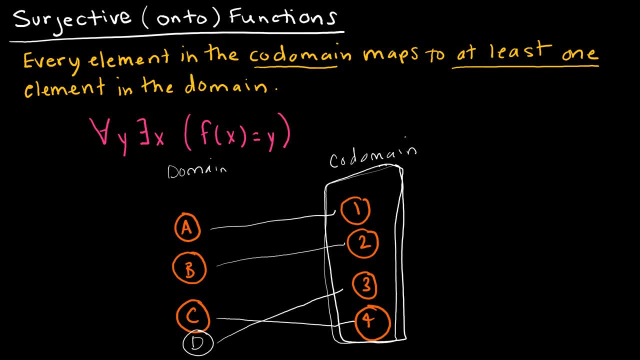 same in this case is mapped to by one element in the domain And it is onto because each element in the codomain is essentially being used, So each element is mapped to. Now let's say, I get crazy and add an element e that maps to one. Well, this is still. 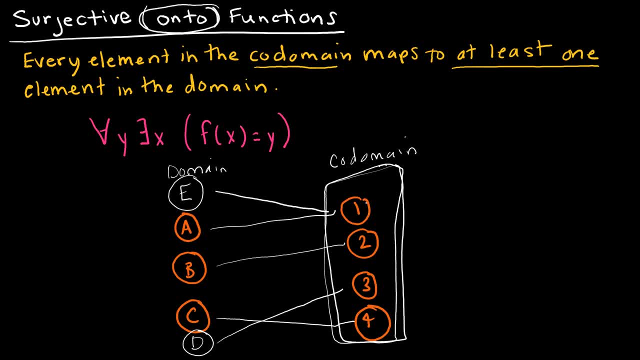 an onto function because every element in my codomain- one, two, three and four- maps to at least one element in the domain. However, by adding this e, I have now made it not a one-to-one function, because one is mapped to by both a and e, So hopefully that helps clear. 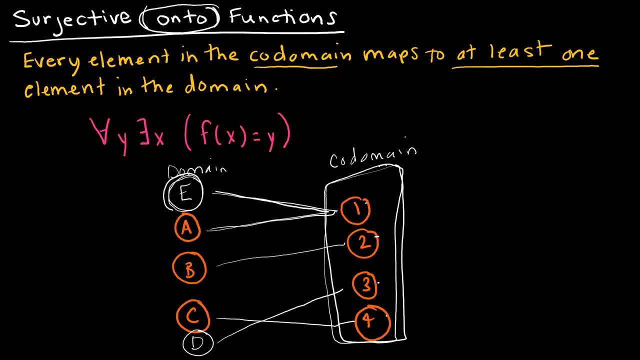 the difference between a one-to-one and an onto function. And again, what this means in propositional logic is: for all y's- these are the y's, the codomain for all y's- there exists some x, such that that x maps to that y. If we happen to have a function that is both. 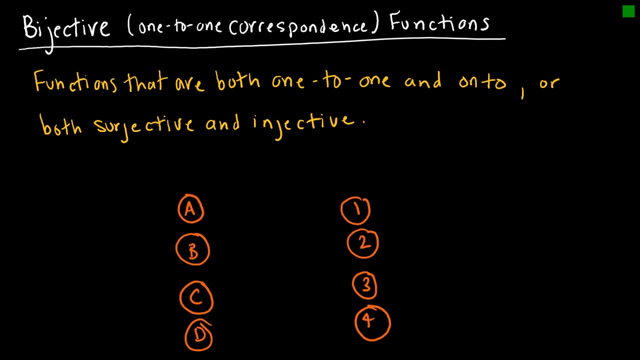 surjective and injective, or both one-to-one and onto. we call that bijective. you might also see it called a one-to-one correspondence. So that means they are both one-to-one and onto. That would mean essentially that each element of the domain is mapped to exactly one element. 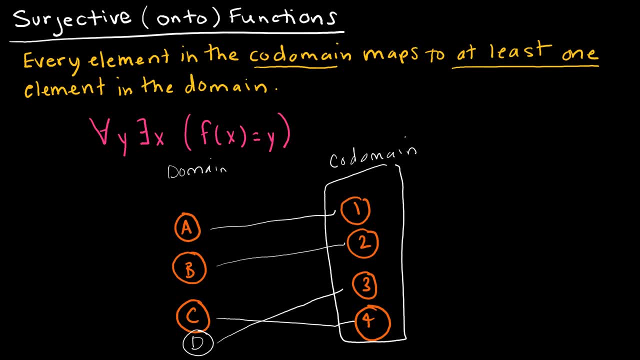 So it's one-to-one because each element here in the range- and the range and the co-domain are the same in this case- is mapped to by one element in the domain And it is onto because each element in the co-domain is essentially being used. 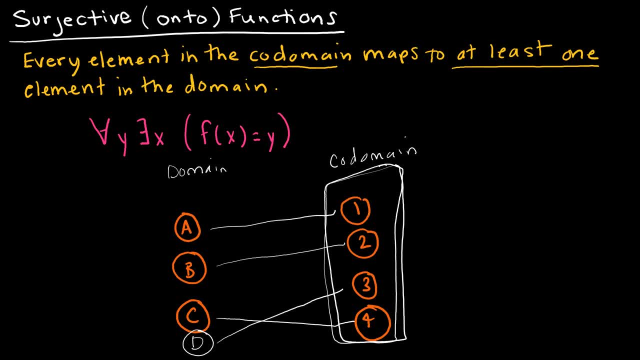 So each element is mapped to. Now, let's say, I get crazy and add an element e That maps to one. Well, this is still an onto function because every element in my co-domain- one, two, three and four- maps to at least one element in the domain. 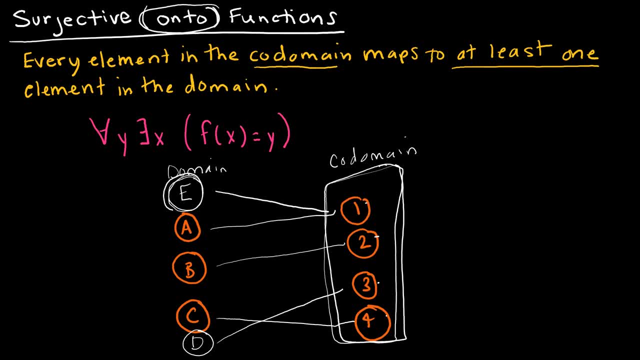 However, by adding this e I have now made it not a one-to-one function, because one is mapped to by both a and e. So hopefully that helps clear up the difference between a one-to-one and an onto function. And again, what this means in propositional logic is for all y's. 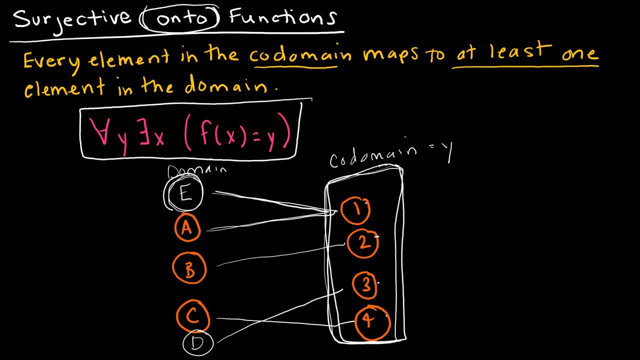 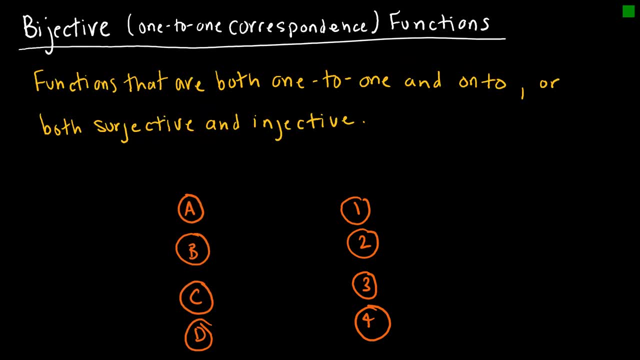 these are the y's, the co-domain for all y's. there exists some x, such that that x maps to that y, If we happen to have a function that is both surjective and injective, or both one-to-one and onto. 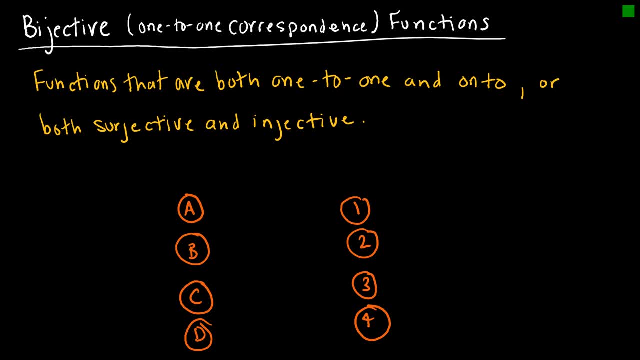 we call that bijective, or you might also see it called a one-to-one correspondence. So that means they are both one-to-one and onto. That would mean essentially that each element of the domain is mapped to exactly one element in the co-domain. 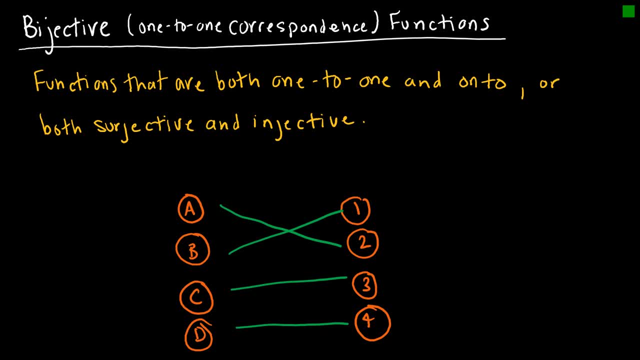 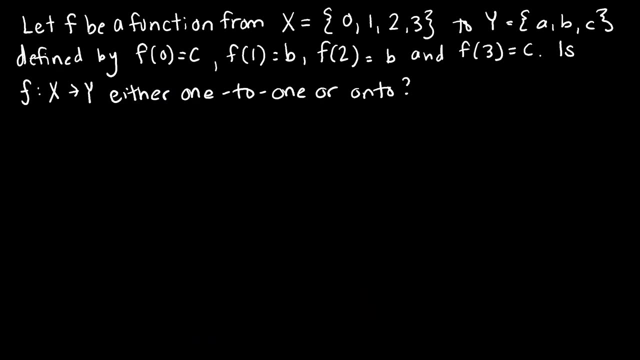 and that there are no elements in the co-domain that aren't mapped to from an element in the domain. So essentially nothing here that's out here by itself, and only one line, only one mapping from each element of the domain. So let's do a practice now to see if we know what we are talking about. 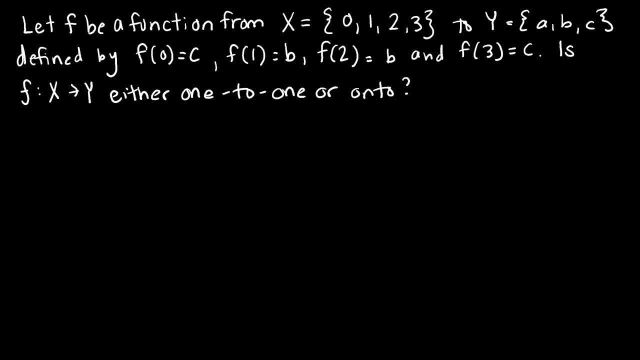 We said: let f be a function from x to y. and again, this is how we would write that. Let me change my colors up a little bit. f is a function from x to y and this is an explicit function, so it's telling me exactly what goes where. 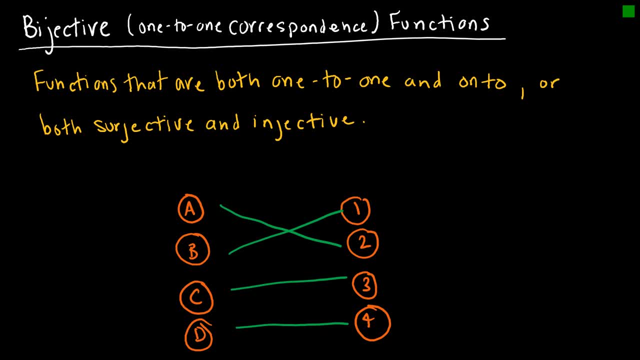 in the codomain and that there are no elements in the codomain that aren't mapped to from an element in the domain. So essentially nothing here that's out here by itself, and only one line, only one mapping from each element. 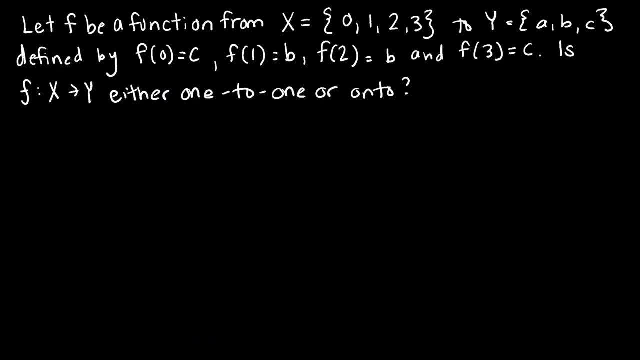 of the domain. So let's do a practice now to see if we know what we are talking about. We said: let f be a function from x to y. and again, this is how we would write that. Let me change my colors up a little bit: f is a function from x to y and this is an explicit function. so it's telling. 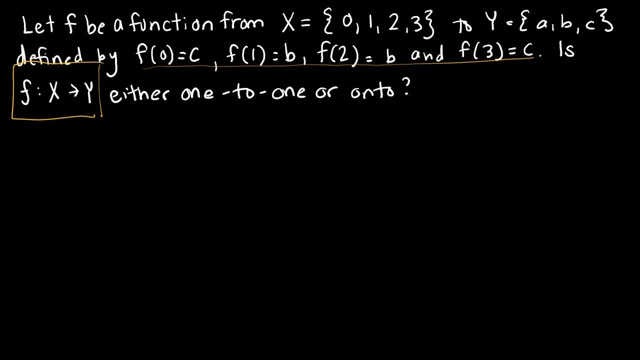 me exactly what goes where. and the question is: is this function one-to-one or onto both? neither, etc. So let's do a mapping, because that to me, is a great, just visual way to see what's going on. So, if x is 0,, 1,, 2,, 3, 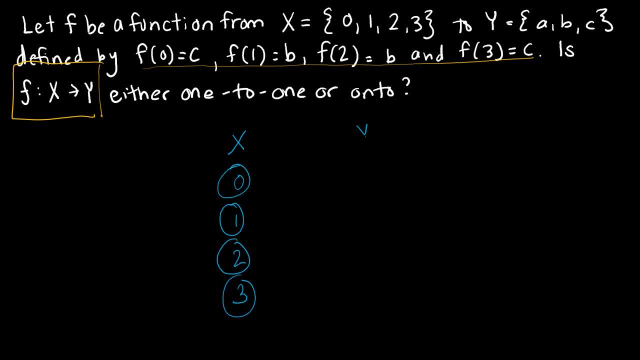 and y is the elements a, b, c, and then I'm going to use f of 0 equals c, f of 1 equals b, f of 2 equals b and f of 3 equals c. So now let's go about answering our questions. Is this function? 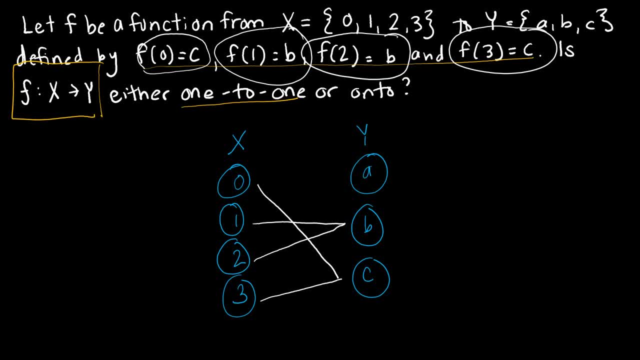 one-to-one? If the function was one-to-one, then each element of the range, so b and c, would have to be mapped to by only one element of x. Is that the case No b is mapped to by both 1 and 2,. 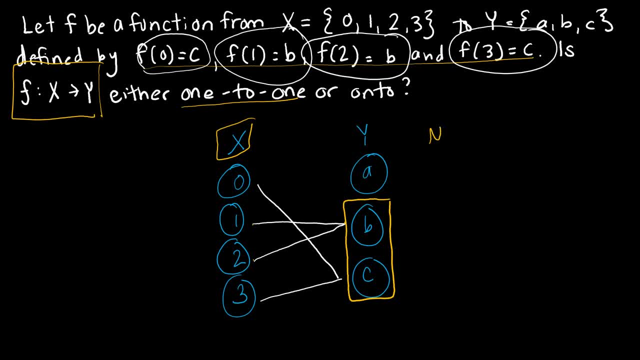 c is mapped to by both 0, and 3.. So this is not one-to-one. Now let's look at onto. If something is onto, then we would expect every value in the co-domain to be mapped to. So I've got a problem with a because a isn't mapped to by anything. So remember. 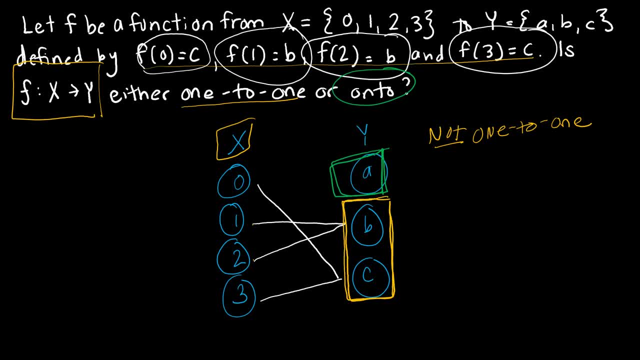 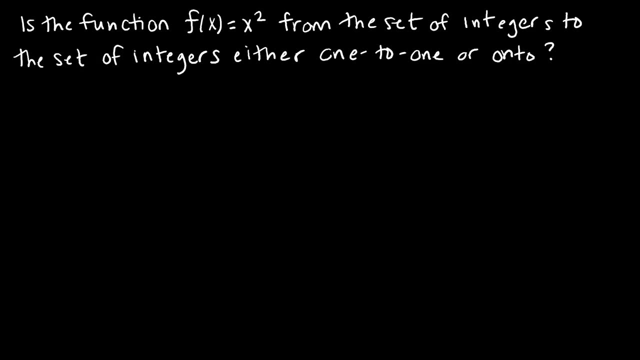 what I've outlined here in yellow is the range, not the co-domain. the co-domain is everything in y, and because I have an element of y that isn't mapped to by an element of x, this is not onto. One more practice for us to try together. This one says is the: 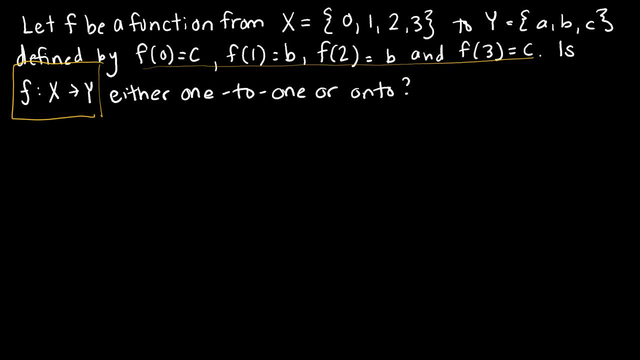 And the question is: is this function one-to-one or onto both? neither, etc. So let's do a mapping, because that to me is a great, just visual way to see what's going on. So, if x is 0,, 1,, 2,, 3,, 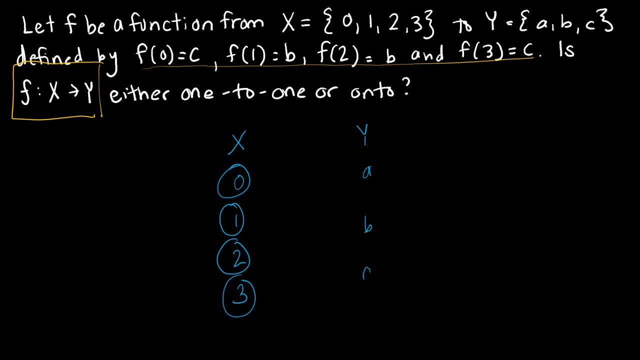 and y is the elements a, b, c, and then I'm going to use f of 0 equals c, f of 1 equals b, f of 2 equals b and f of 3 equals c. So now let's go about answering our questions. 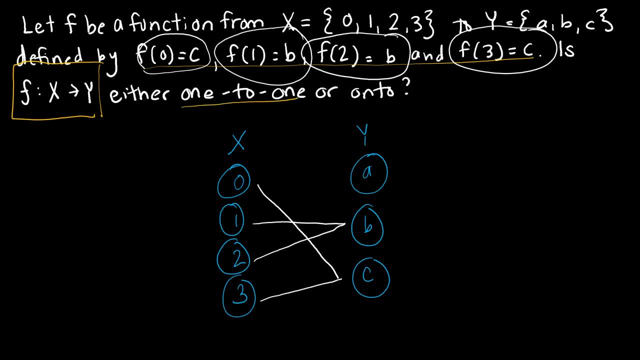 Is this function one-to-one? If the function was one-to-one, then each element of the range, so b and c, would have to be mapped to by only one element of x. Is that the case? No b is mapped to by both 1 and 2,. 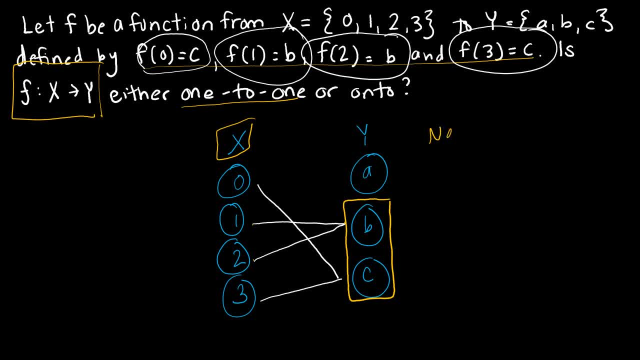 c is mapped to by both 0 and 3, so this is not one-to-one. Now let's look at onto. If something is onto, then we would expect every value in the codomain to be mapped to. So I've got a problem with a. 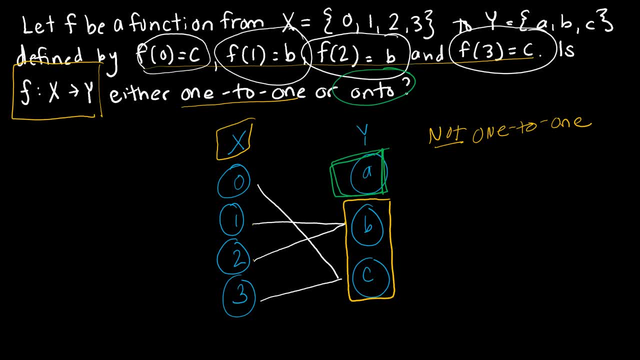 because a isn't mapped to by anything. So remember, what I've outlined here in yellow is the range, not the codomain. The codomain is everything in y and because I have an element of y that isn't mapped to by an element of x. 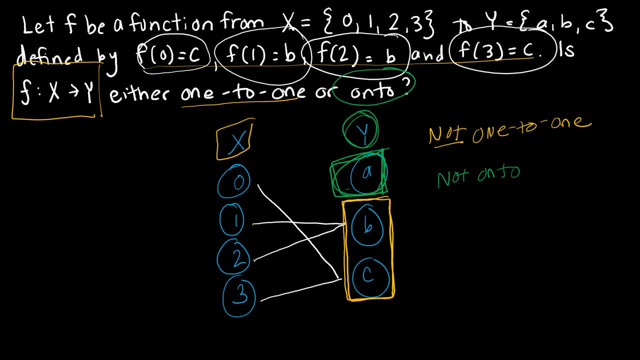 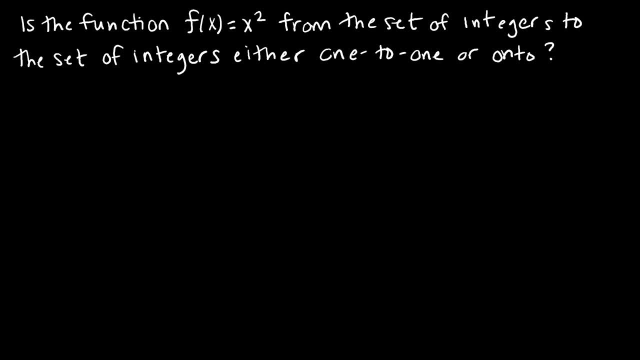 this is not onto. One more practice for us to try together. This one says: is the function f of x equals x squared from the set of integers to the set of integers, either one-to-one or onto and again, or neither or both. 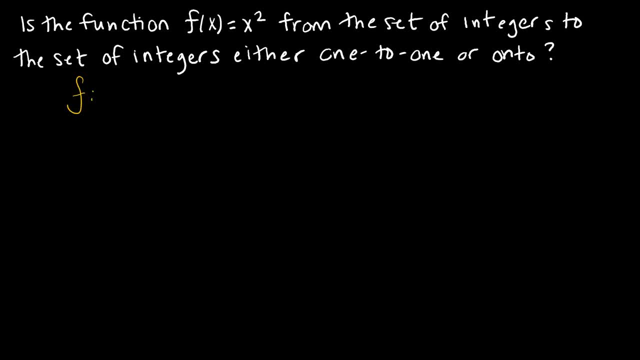 So again, just as a side note, you might see it written like this, where I'm saying f is a function from the integers to the integers, And again we're asked to show: is it one-to-one or is it onto? 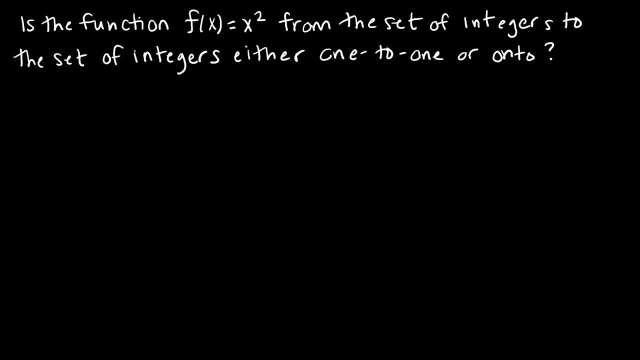 function f of x equals x squared from the set of integers to the set of integers, either one-to-one or onto and again, or neither or both. So again, just as a side note, you might see it written like this, where I'm saying f is a function from the integers to the integers, and again we're asked: 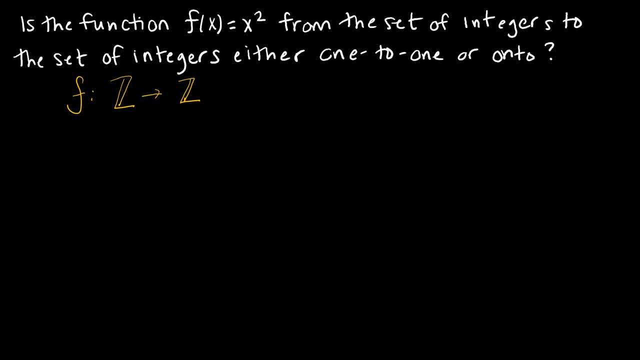 to show. is it one-to-one or is it onto? Now, this one's a little bit harder, because we don't have, just, you know, a set of discrete elements. These are continuous sets, all of the integers, and I would start by looking at one-to-one. 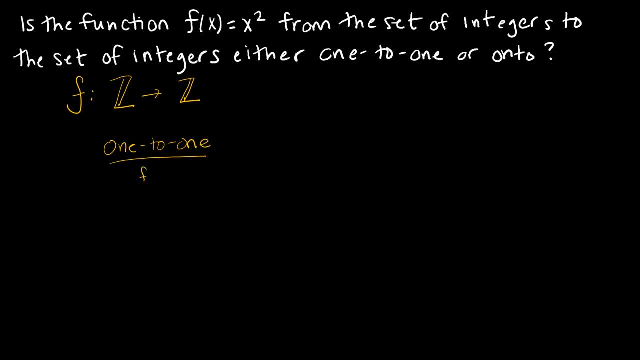 So if you recall for it to be one-to-one, we're saying, if a, f of a is equal to f of b, then it must imply that a is equal to b. That was one of the ways we talked about to show one-to-one. So let's say again, looking at this function: what if a was 2 and b was negative 2.. 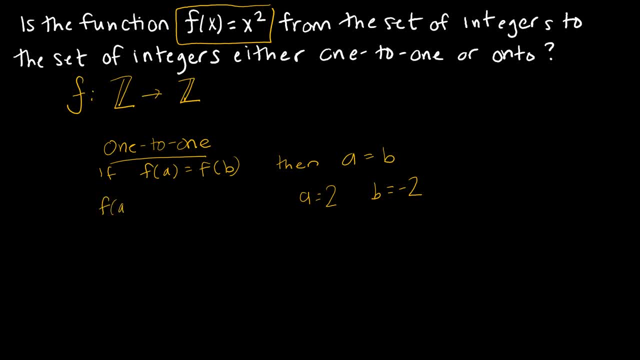 2.. Then f of a would equal 2 squared 2 times 2,, which is 4.. And f of b would equal negative 2 times negative 2, negative 2 squared, which is 4.. So I can say in this case that f of 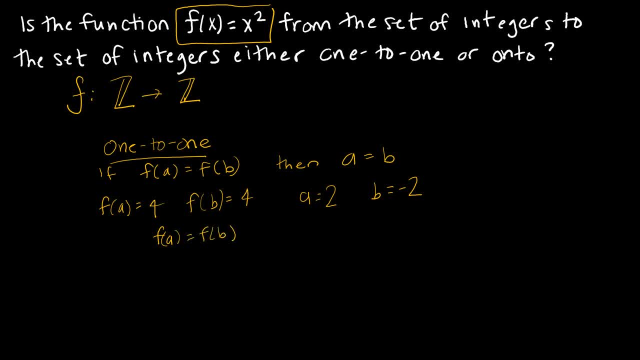 a is equal to f of b, but a does not equal b. therefore, this is not 1 to 1.. So now let's take a look at onto. Onto says: if you have a value in your codomain, it must be mapped. 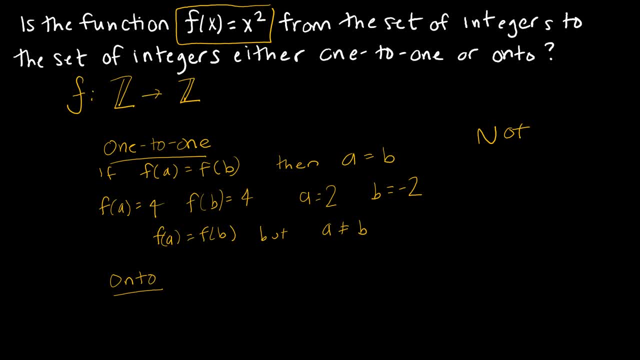 to by an element in the domain. So remember, the domain is all integers, the codomain is all integers. Am I ever going to get a value for my codomain, which is what happens when I square x? Is that ever, ever, ever, ever going to be say negative 1? Can I ever square? 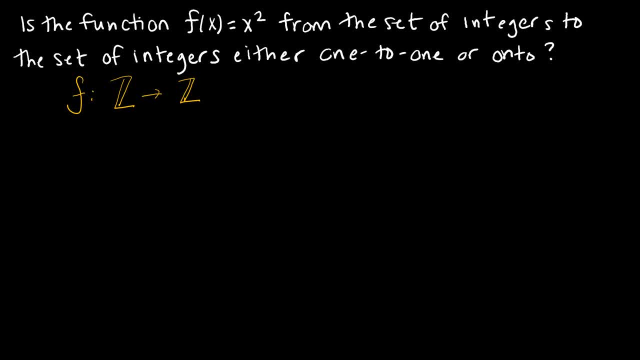 Now, this one's a little bit harder because we don't have just a set of discrete elements. these are continuous sets, all of the integers, And I would start by looking at one-to-one and if you'll recall for it to be one-to-one, 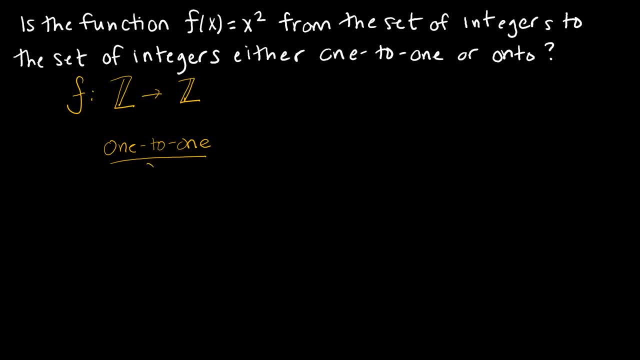 we're saying if f of a is equal to f of b, then it must imply that a is equal to b. That was one of the ways we talked about to show one-to-one. So let's say again, looking at this function: 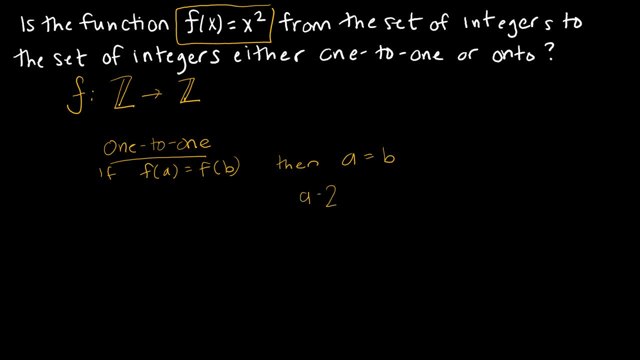 what if a was two and b was negative two? Then f of a would equal two squared two times two, which is four, and f of b would equal negative two times negative, two negative two squared, which is four. So I can say in this case that f of a is equal to f of b. 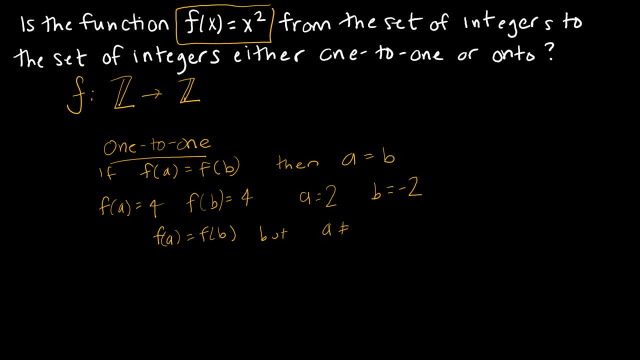 but a does not equal b, therefore this is not one-to-one. So now let's take a look at onto. Onto says: if you have a value in your codomain, it must be mapped to by an element in the domain. 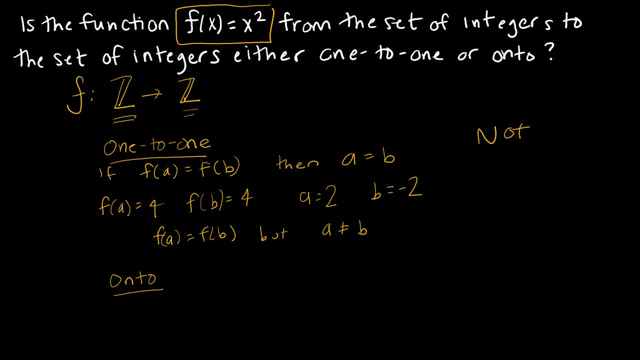 So remember, the domain is all integers, the codomain is all integers. Am I ever going to get a value for my codomain, which is what happens when I square x? is that ever, ever, ever, ever going to be? 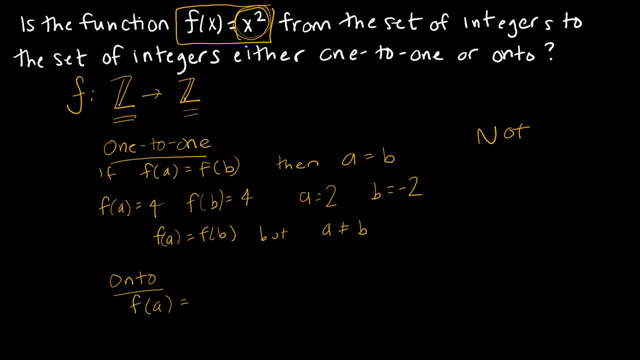 say negative one. Can I ever square an integer and get negative one? No, I can't. So because I have some value, there exists some value, then this is not a one-to-one function, because this guy, and along with every other negative value, 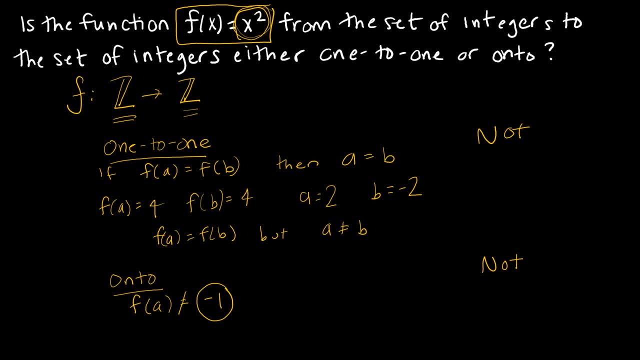 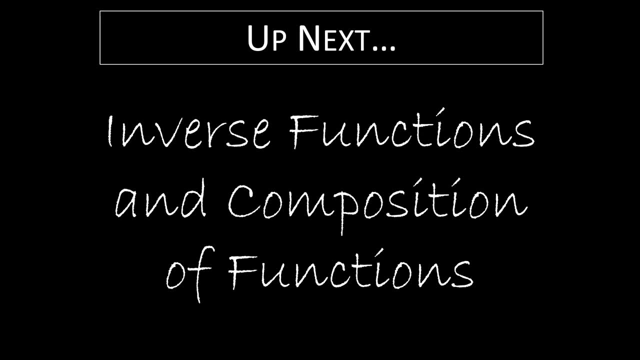 is not ever going to be in the range Coming up. next we're going to take a look at inverse functions and composition of functions.